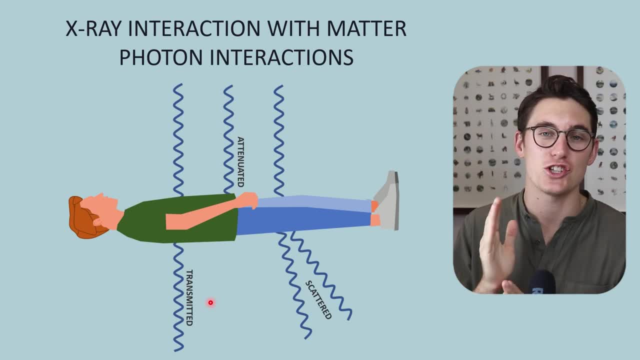 with this x-ray and the tissues itself. There has been no energy deposited here. that x-ray has gone through unscathed, reaching our x-ray detector. The second thing that can happen is x-ray beam attenuation, absorption of that x-ray Without any x-ray reaching our detector, and this is the process. 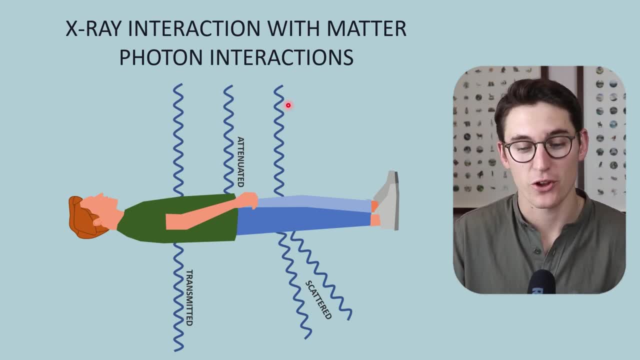 of the photoelectric effect that we're going to look at today. The third interaction that can happen is what is known as scattering here, where our incident x-ray is deflected at an angle, either through the Compton scatter or Rayleigh scatter interactions. So today let's start by looking at 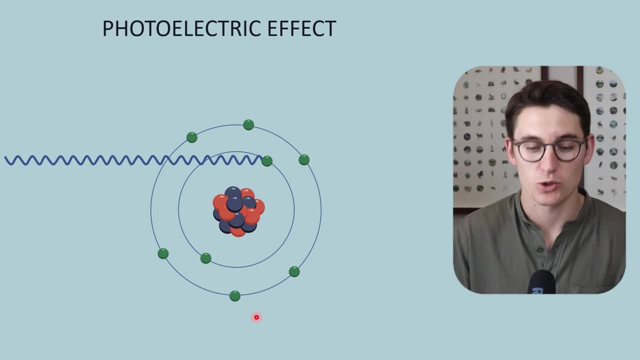 attenuation here, or the photoelectric effect. So what exactly is the photoelectric effect? Well, we have an atom here, within our tissues, within the patient that we're imaging, And this is the incident: X-ray beam that's coming from our X-ray tube. 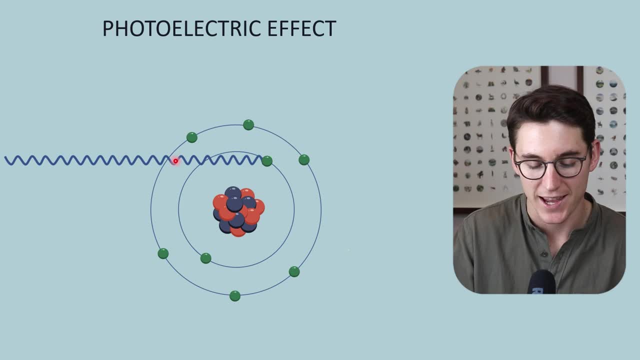 It's either Bramstrang or characteristic X-ray radiation heading towards the patient tissue. Now what happens is this X-ray will collide with an electron within that atom And all of that X-ray's energy will be deposited into that electron. The entire X-ray energy has been annihilated there. 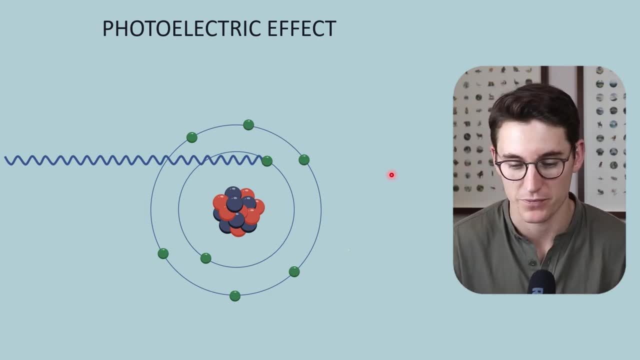 All of that energy is now being conferred onto this electron. That electron will then be released if this energy of this incident X-ray- is higher than the binding energy of that electron. If it's higher than the binding energy, that electron is released. And the release of that electron 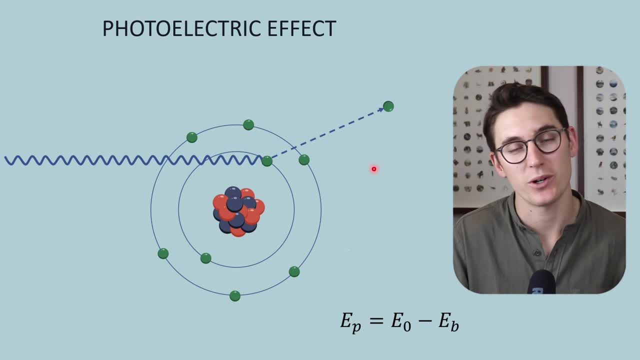 is what's known as a photoelectron, And it's this photoelectron that is traveling through the patient's tissue that is going to confer the most dose to the patient. You see, when an X-ray travels through a tissue, it only interacts when it comes. 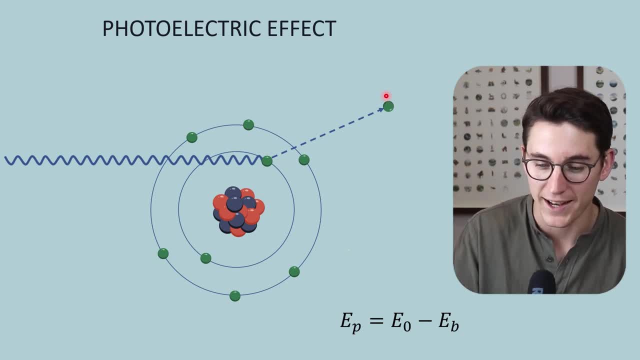 into a direct collision like this, When an electron travels through a tissue because it's negatively charged. an X-ray has not got any charge, but an electron does, because it's negatively charged. it can repel surrounding electrons And that is how we infer dose onto the patient. 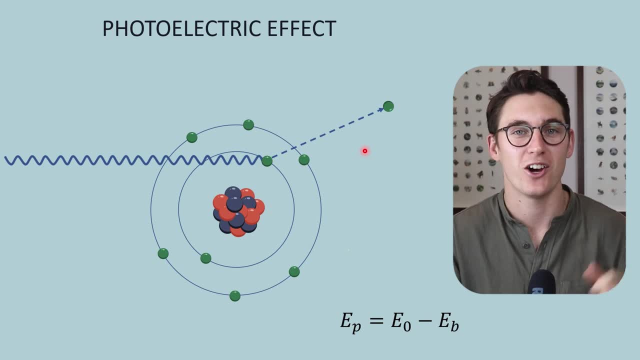 through a process known as linear energy transfer, which we're going to look at after these three lectures. So, what energy transfer is this? What energy does this photoelectron have? Well, we can use this formula: The energy of the photoelectron is equal to the incident energy of our X-ray. 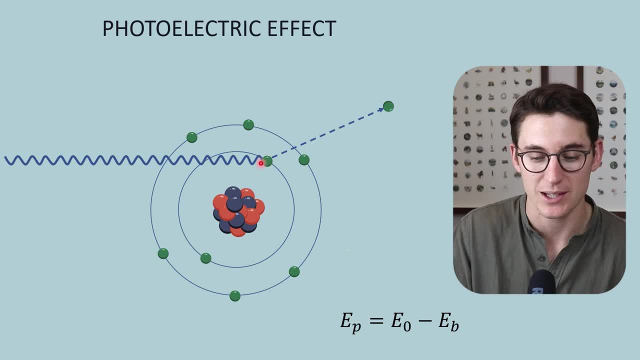 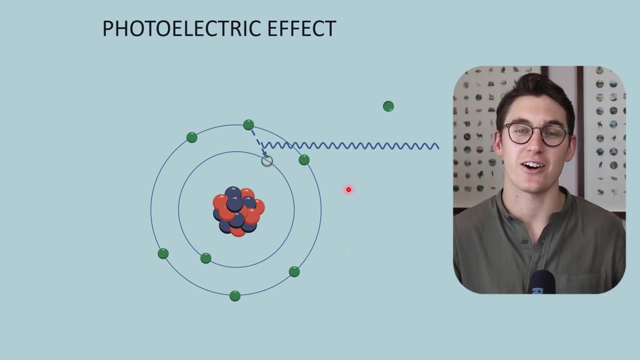 minus the energy required to release that electron, the binding energy of that electron. So this photoelectron has the energy of this incident X-ray minus the binding energy of that electron. Now we've created a vacancy here And, as we've seen in our characteristic radiation production, talk. 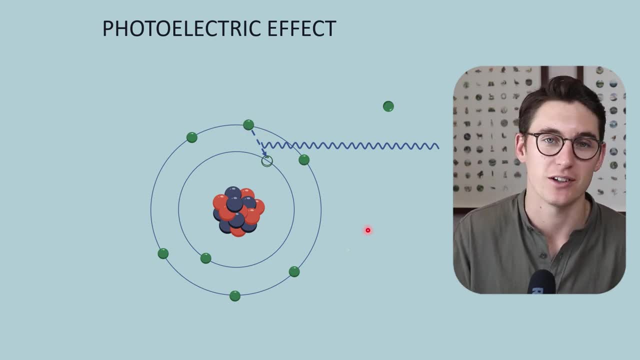 that vacancy will be filled by an outer shell electron. So here an L-shell electron is dropping down from a higher energy state to a lower energy state, And that loss in energy is released in the form of a characteristic X-ray. So you may be wondering. 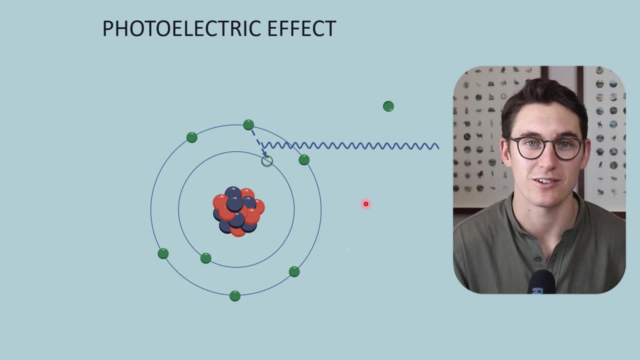 doesn't this characteristic X-ray then go off and head to our detector? And that is a valid thought? but there is a reason: this characteristic X-ray will never reach our detector. When we looked at characteristic X-ray. when we looked at characteristic X-ray- 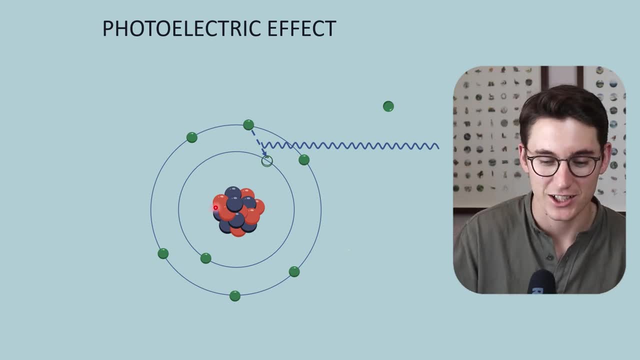 X-ray production. our target material was tungsten. It had an atomic number of 74.. When we're dealing with tissues- X-rays interacting with matter within a patient- our average atomic number is seven. The binding energies here are much, much lower. 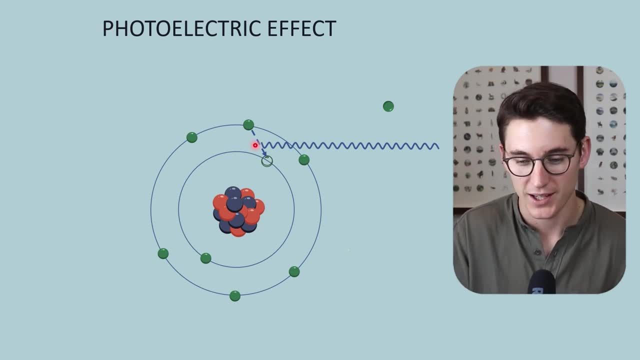 in patient tissue as opposed to our anode target material. And we know this characteristic X-ray being released is the difference between the binding energy of our K and our L-shell electrons. Here this energy of this characteristic X-ray is very, very small, less than one keV. 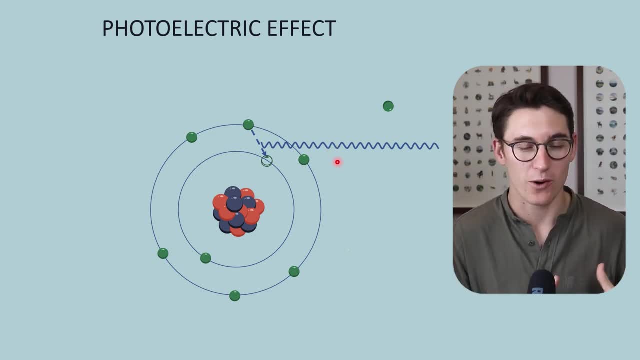 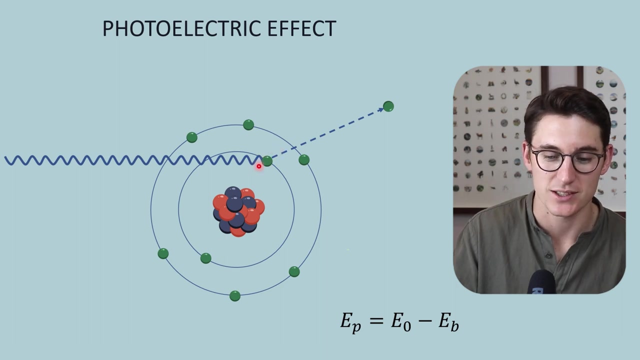 And that X-ray will be attenuated within the patient's tissues and won't be able to reach the detector. So the photoelectric effect differs from characteristic X-ray production in a couple of ways, The most importance of which is that the photoelectric effect has an incident X-ray that releases an electron. 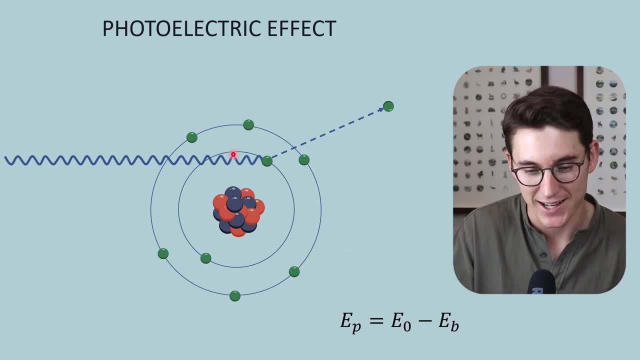 In characteristic X-ray production at the anode. it's an incident electron that is releasing this electron from our K-shell. So we've created an ion here. Our atom has one less electron than it had previously. We've created a low energy X-ray. 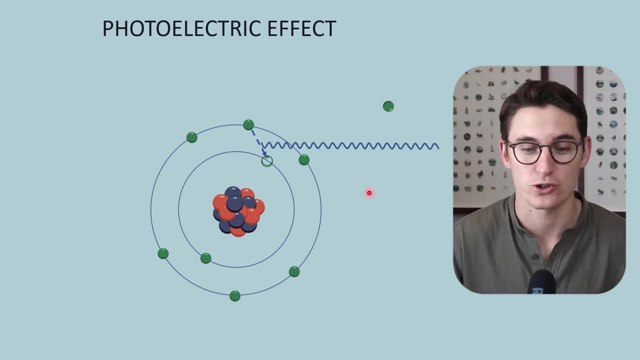 and we've created a photoelectron that is gonna confer dose to our patient. Now, what is the probability of the photoelectric effect to occur? Now, we've looked at this before when we looked at X-ray beam filtration, when we preferentially removed lower energy X-rays. 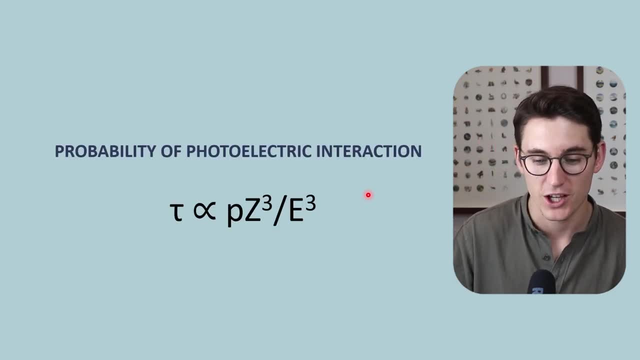 by adding a filter in our Brems-Lang curve And we looked at this formula here: the probability of a photoelectric interaction to occur. This probability is proportional to the density of the patient's tissue, the atomic number of that tissue to the power of three. 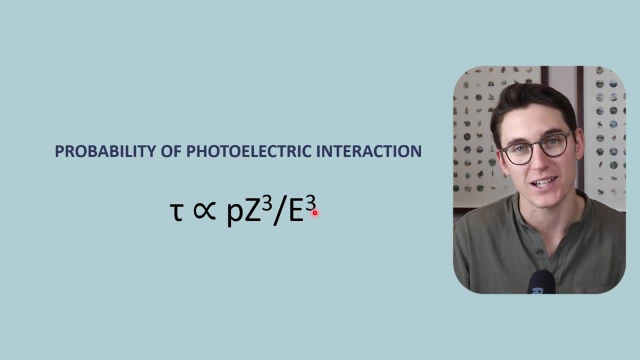 and it's inversely proportional to the energy of that incident X-ray coming towards our patient. So the denser a tissue, the more likely that X-ray beam is to be attenuated. If we look at bone, bone costs a shadow, a beam, a beam. 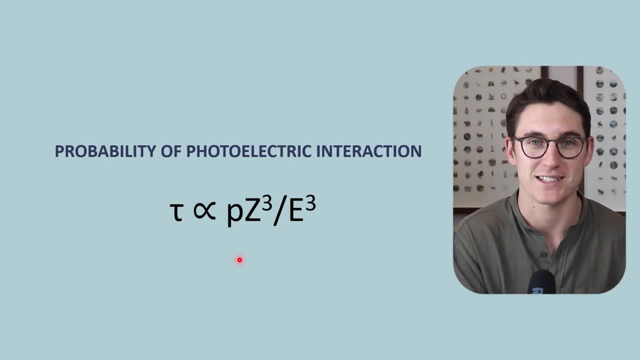 and a quick-release force. we can see that bone costs a shadow on our X-rays because more photoelectric effect is happening there. The higher our atomic number, the higher the probability of the photoelectric effect to occur is. When we give contrast iodine, it has a high atomic number. 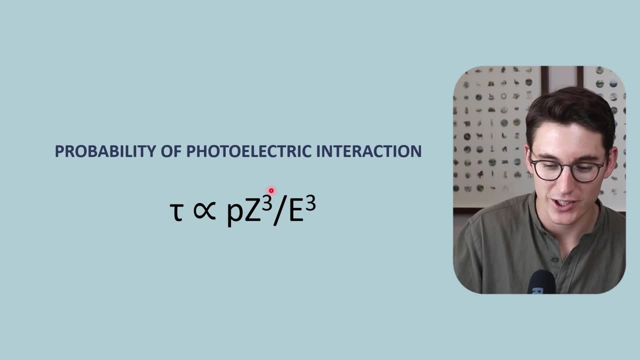 We get a big shadow cost on our X-ray there. because that high atomic number of the iodine is increasing, the likelihood of the photoelectric effect to occur Now perhaps counter-intuitively increases. we get less and less photoelectric effect occurring. Now, the way I like to think, 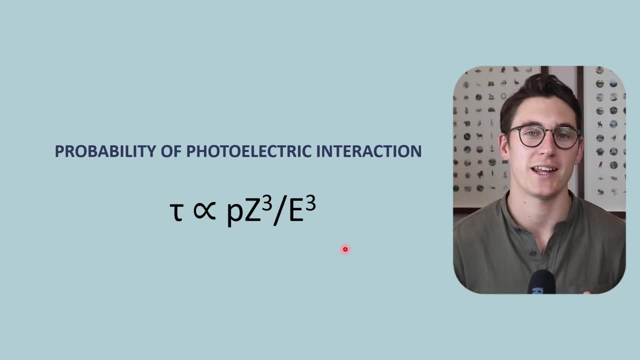 about x-ray energies interacting with matter is by way of an analogy. Now, if you've ever looked at a ceiling fan, if you've been in a hotel, and there's that fan on the ceiling and the blades are rotating at a set speed. think of those blades as the electrons rotating around our atoms within. 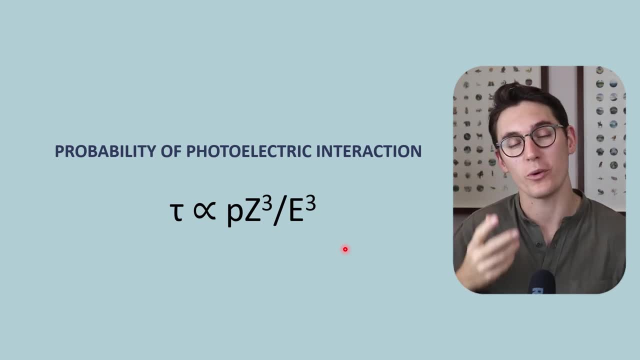 the patient's tissue. Now if I was to hold the ball and throw it towards that fan, think of the ball as the incident x-ray heading towards our patient's tissue. The slower I throw that ball towards the fan, the more likely that ball is to hit one of the blades of that ceiling fan. The faster and faster. 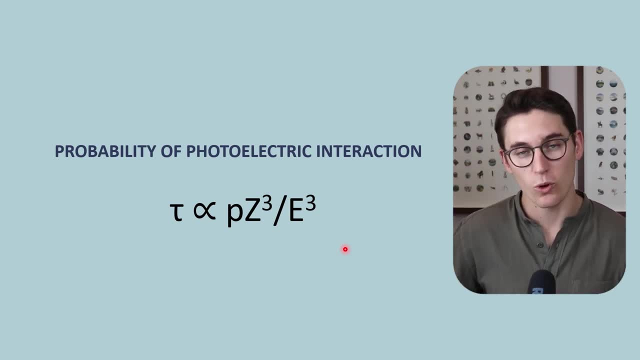 I throw that ball. the higher and higher that x-ray energy, the more likely it is to miss the blades of the fan and hit the ceiling. The same happens here: As we increase our x-ray energies, the less likely it is to hit one of those electrons within our target material. Now we can represent this. 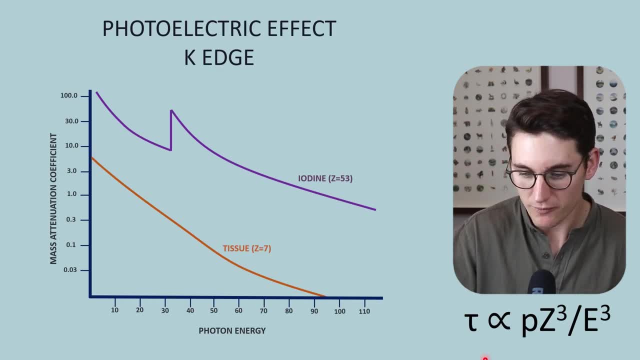 graphically and we can see that in tissue here, as the photon energy increases of our incident x-ray, the likelihood of the photoelectric effect to occur decreases. And you can see our mass attenuation coefficient on the y-axis of our graph. This is something we're going to go over. 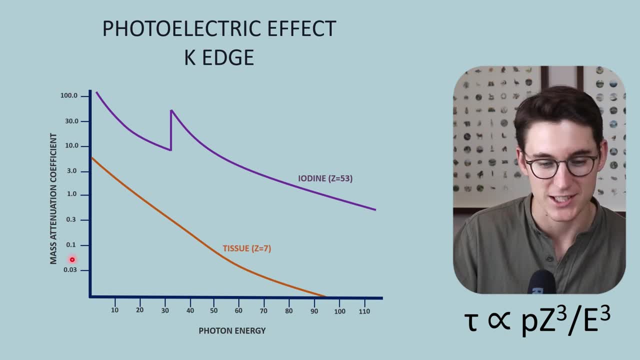 in a future talk. This is an exponential change on this axis. So, although this looks quite linear, this decrease, this is actually an exponential decrease in the likelihood of the photoelectric effect to occur. Now you can see here I've included iodine with a higher atomic number. We see that atomic number to the power of 3. 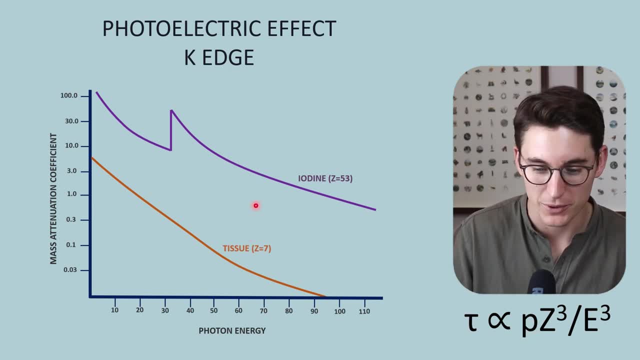 increases the likelihood of the photoelectric effect to occur. Because iodine's atomic number is so much higher, the likelihood of the photoelectric effect to occur is so much higher. Now you may be wondering what is the strange jump within the iodine here? and this is what's known as the k edge. 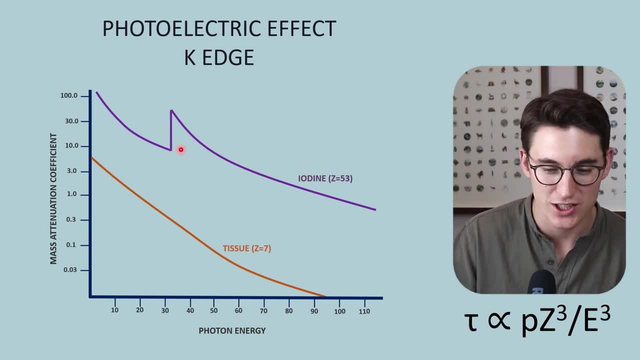 Now, what is the k edge? Well, the k edge is the energy level at which our k-shell electron within the iodine iodine here will be released- the binding energy of our K-shell electron. At energies below that range we cannot release that K-shell electron, so we are not getting the photoelectric effect. 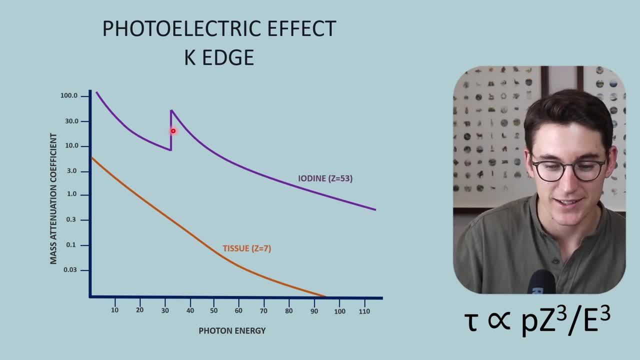 occurring there, As our X-ray energies are higher than that K-shell binding energy. we then make available a whole load more electrons for the photoelectric effect to occur. We get the sharp increase in the likelihood of our photoelectric effect to occur, and we can use this to our 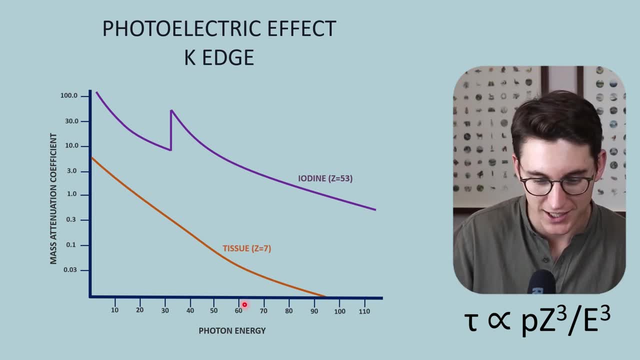 advantage when we use iodine in contrast studies. This is the diagnostic energy range. here We get the benefit of that K-shell or that K-edge occurring, increasing the likelihood of the photoelectric effect to occur, increasing the contrast between our iodine and our surrounding. 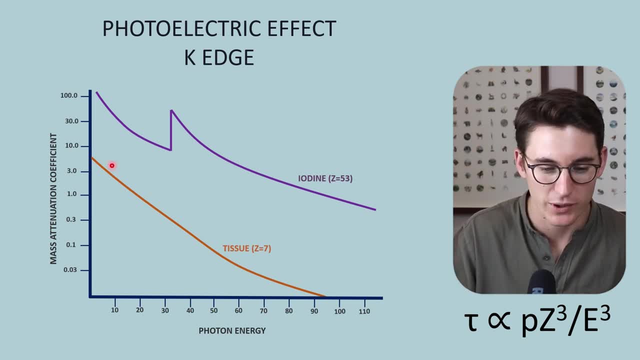 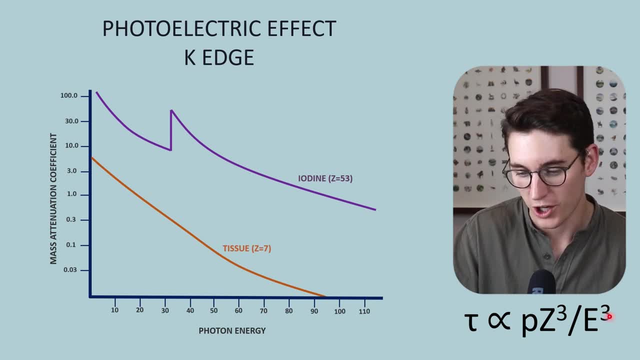 small that we don't see it on this graph. We get this drop off according to this probability formula here, where our likelihood of the photoelectric effect to occur decreases exponentially as photon energy increases. Now this becomes really important to note, especially when we 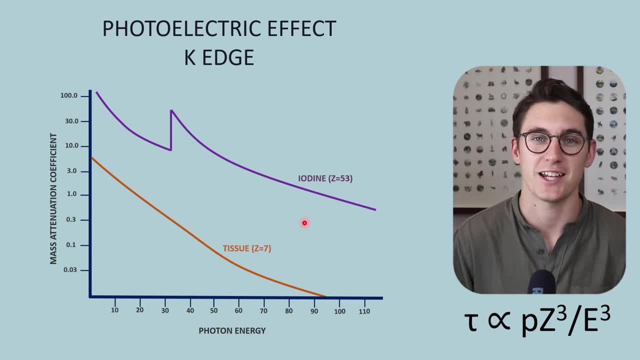 start looking at Compton scatter and Rayleigh scatter in the diagnostic energy ranges, And it's the differences in the density and the atomic numbers of the various different tissues within our body that provides us with the anatomical detail in our image, And in an ideal world we would only want either X-ray transmission or the photoelectric effect to